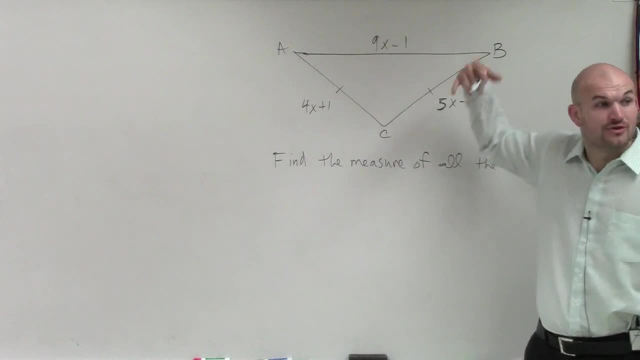 notice right now that this triangle has two side lengths, So therefore we can call this a isosceles, right? So it's an isosceles triangle where these two measures are equal to each other. Now they want us to find the value of each and every side, So we need to find 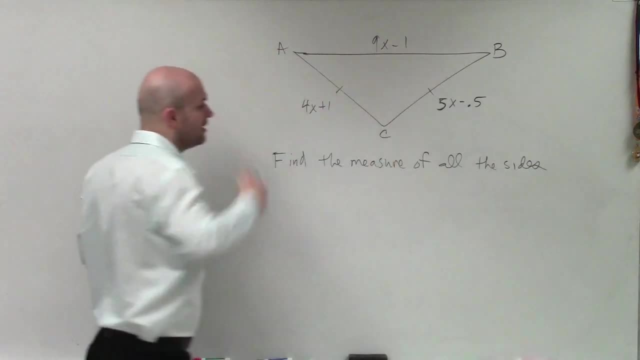 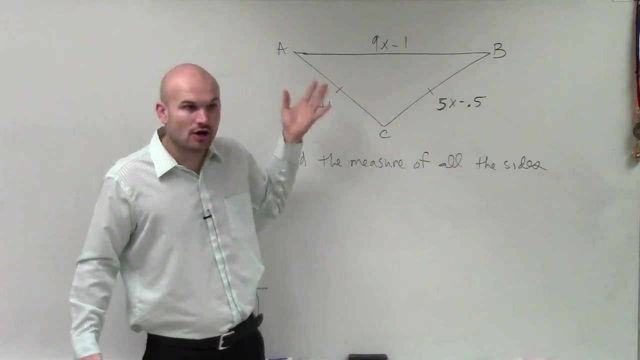 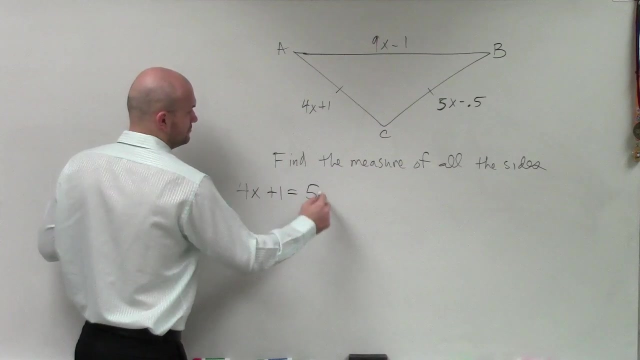 the value of AB, AC and BC for the measurement. So to do that, we need to find the value of X. The only thing we know is that these two sides are equal to each other. Well, if they're equal to each other, therefore, I can set up an equation Again. why can I say they're? 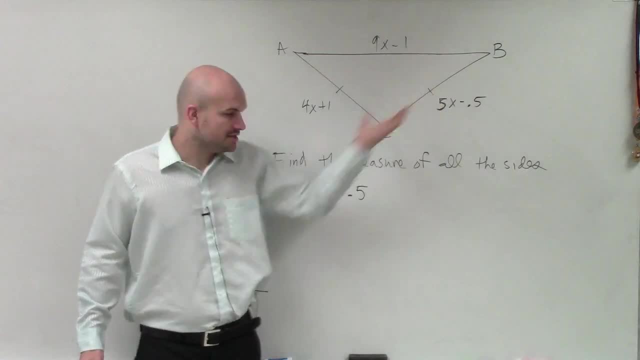 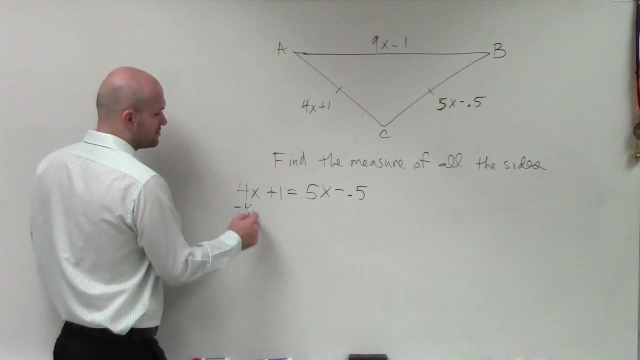 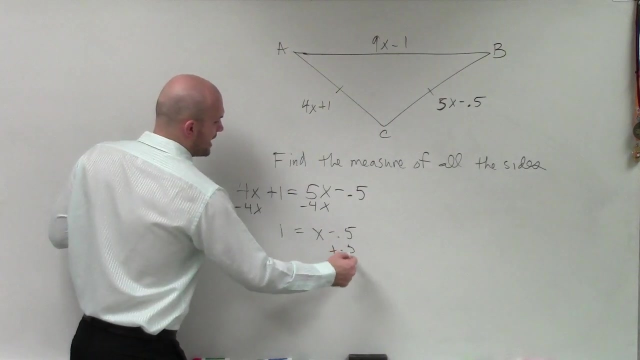 equal to each other Because, remember, these tick marks tell you they're equal to each other. So we can set up an equation. Now I have an equation that I can go ahead and solve. So now I just need to solve for X, So I'll subtract for X, So I have 1 equals X minus 0.5, add 0.5, add 0.5.. Therefore, 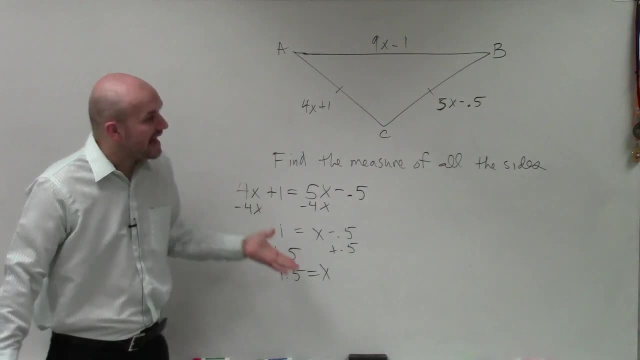 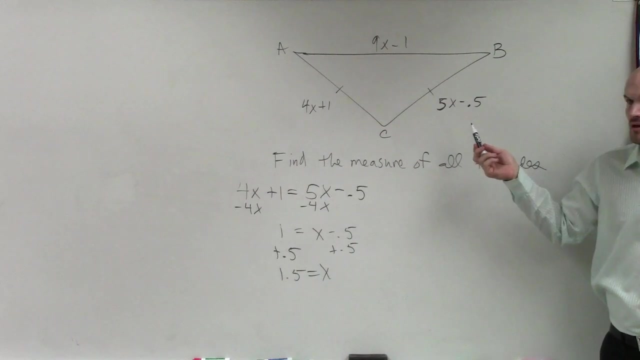 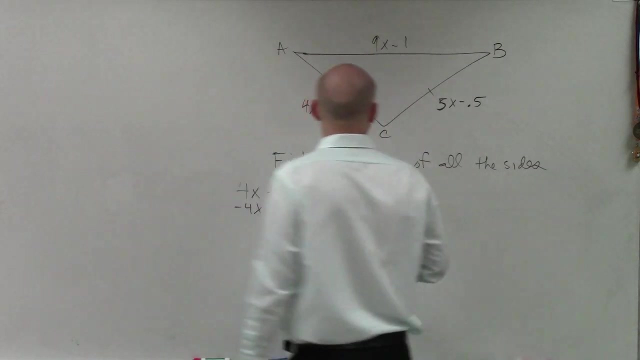 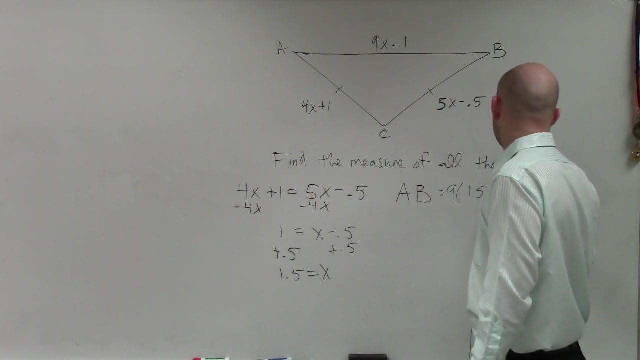 I have: 1.5 equals X. So now that I know the value of X, can I plug in the value of X for each one of these equations to find the length of each one? Yes, I can. So therefore I can say the measurement of side AB is going to be 9 times 1.5 minus. 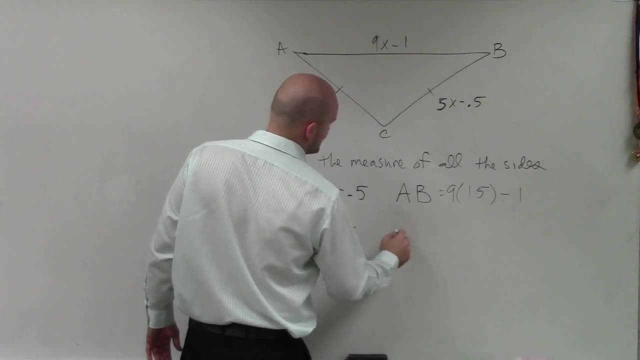 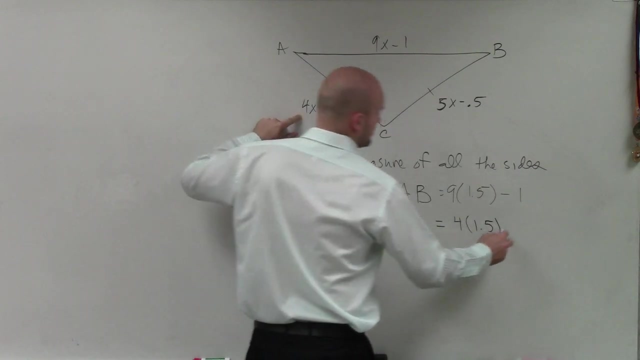 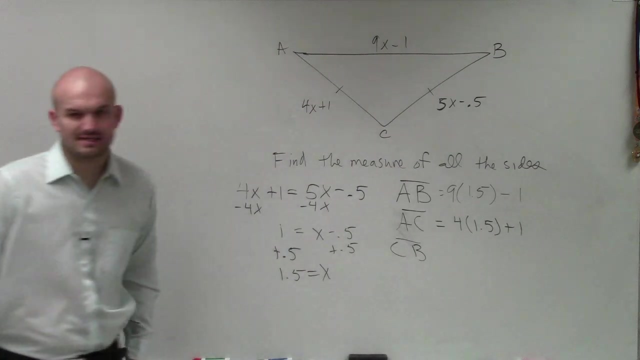 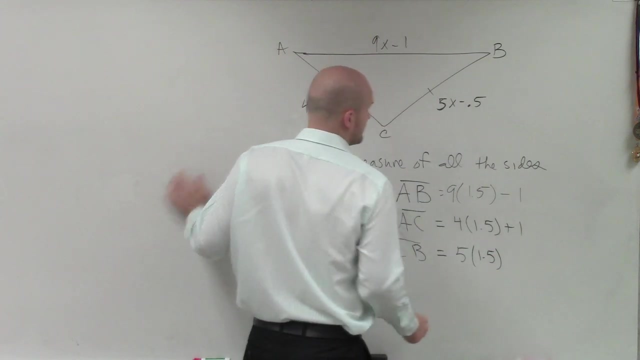 1. Side length AC is going to be 4 times 1.5 plus 1. And side for CB. these are all line segments, right, They're all sides. Line CB is equal to 5 times 1.5 minus 0.5.. 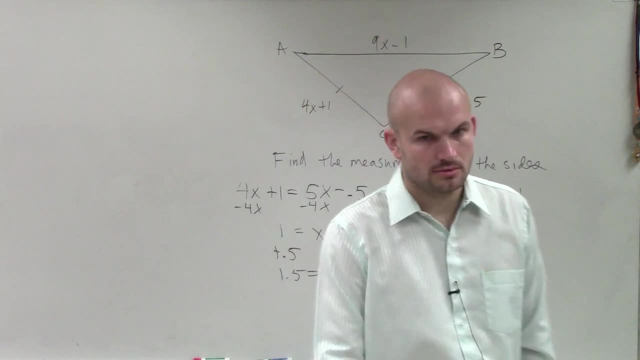 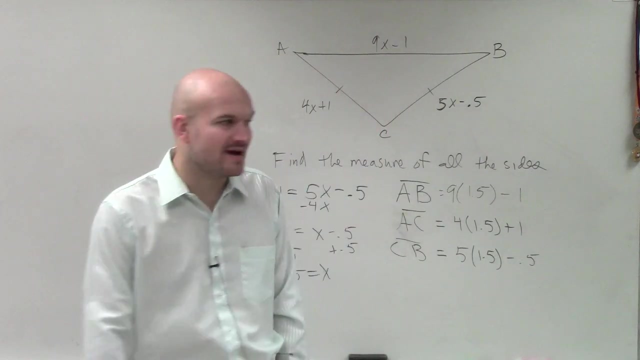 So now I just need to do the work. So 9 times 1 is going to be 9.5 is 4.5, right Half of 9 is 4.5. So that would be 13.5 minus 1 would be 12.5..